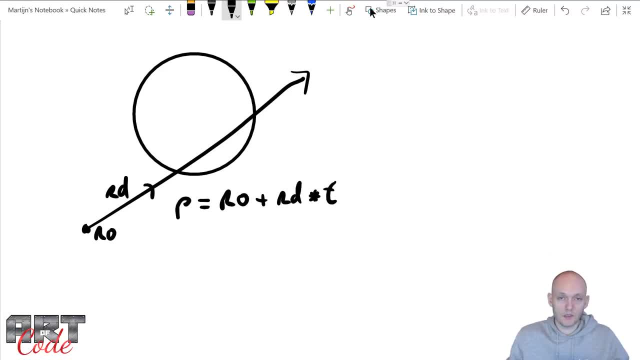 if this time is zero, then my point is just going to be the ray origin plus zero times the ray distance, And if my T increases, then the point will slowly start moving along the ray. All right. So now the question becomes: what is this T1 over here? 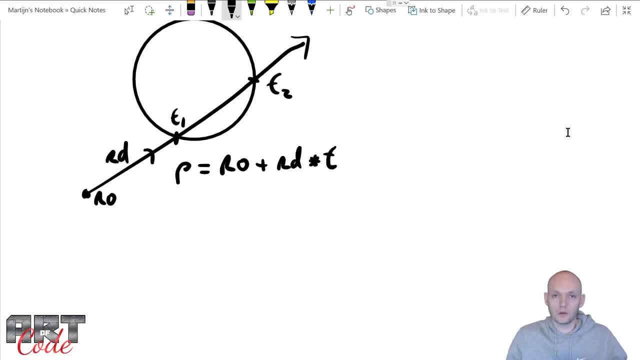 and what is this T2?? So those are the intersection points that we're trying to find. Now let's just first find something else. which is the point? if this is the center of the sphere, let's first try to find the point that is the closest to the center of the sphere. 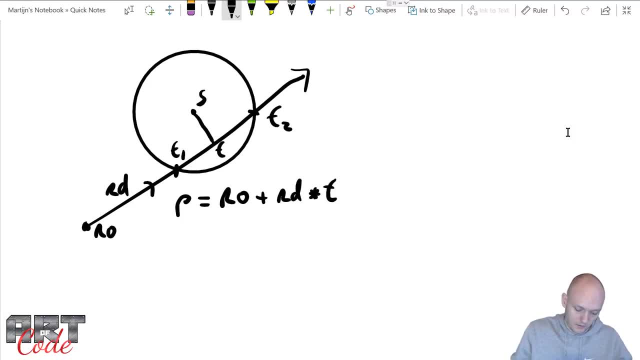 Okay, let's call that point T, All right, so this would be 90 degrees. So that turns out to be so. point T turns out to be the dot product between this ray. Okay, so like it's this vector. 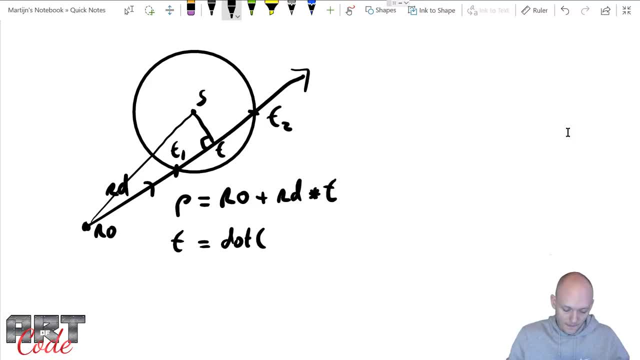 the vector that goes from the ray origin to the center of the sphere and the ray direction. So the first one is S minus RO, which is the vector from the origin to the center of the sphere and the ray direction. All right, so that's my T. 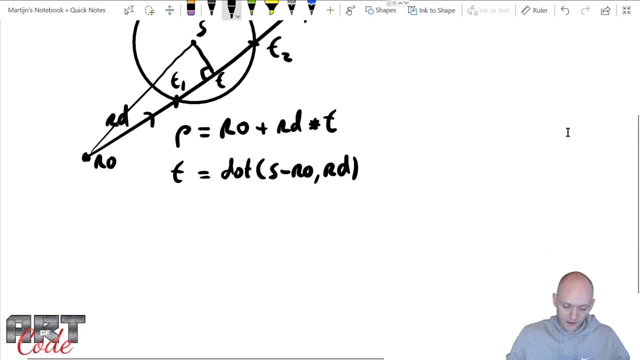 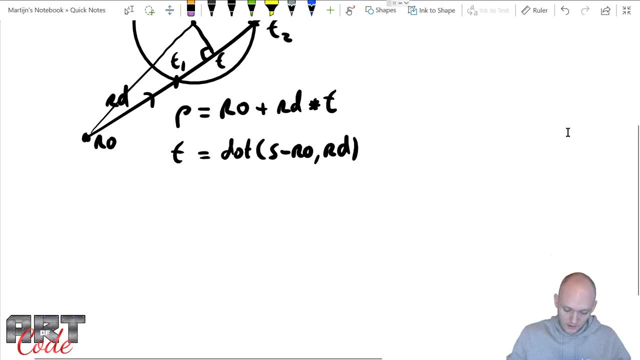 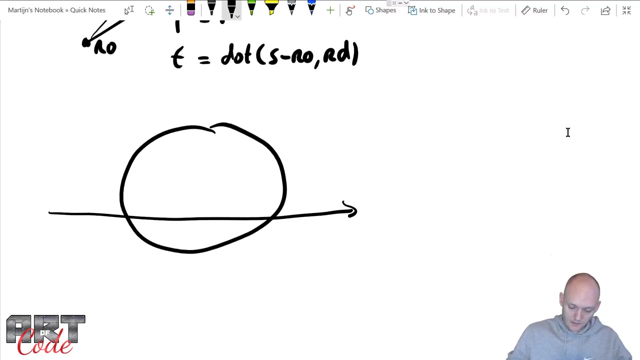 Now let me draw this again And just rotate this so that everything is straight. So let me go over here and give it a bit more space, Not that? All right. well, let me just draw it like this, All right. and now there is my ray. 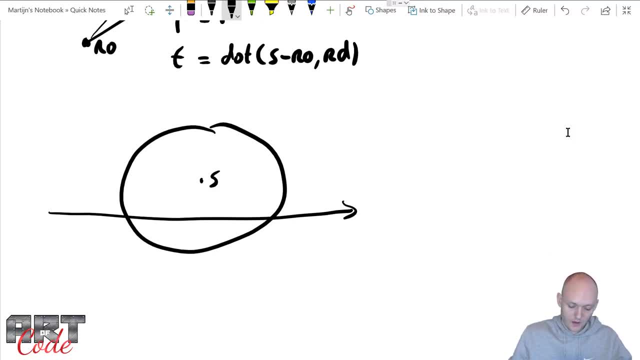 And here is my center of the screen of the sphere, And now we have our T1 over here And our T2 over there, And now our T is over here. And so now what we're interested in is finding this value x here. 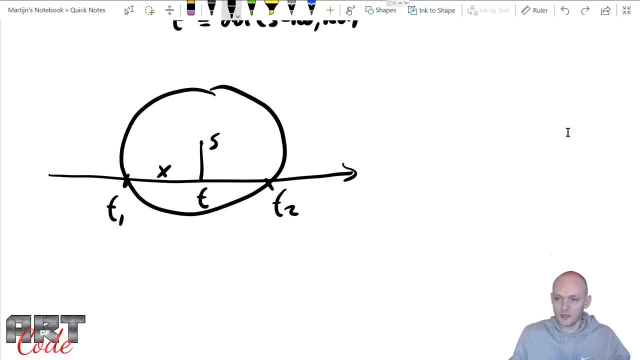 which is the distance between here and here. Right, So well. so let's try to find that x. Well, the x we can find by using the formula for a circle. So the formula for a circle is x squared plus y squared. 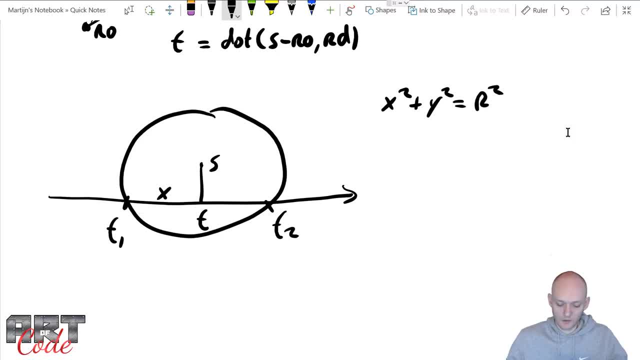 Equals the radius squared, Okay, and the radius obviously is that over there, right, And that's that's given. So if we let's, let's solve this for for x. So what we can do here is like take this y squared, put it on the other side. 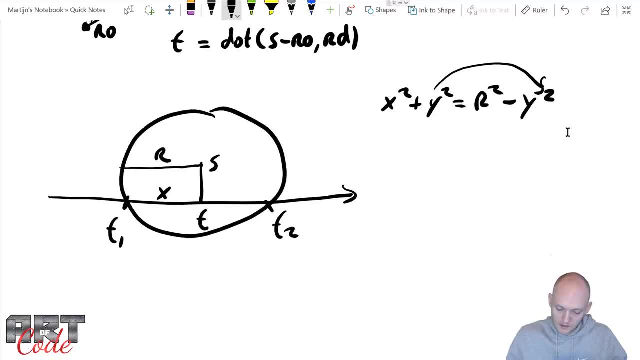 So now I have minus y squared, and that will get rid of all of this. And now we take the, the square root on both sides of the equation, So then I can get rid of this, and then over here I'm just going to have the square root. 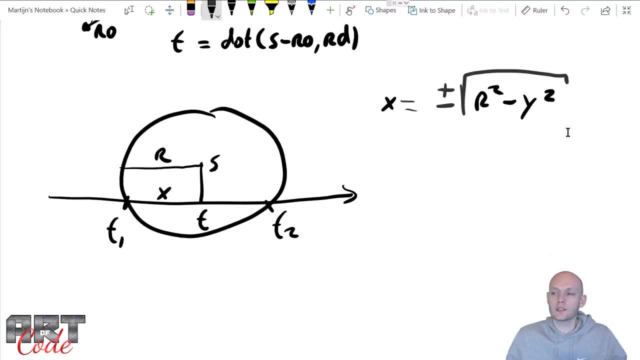 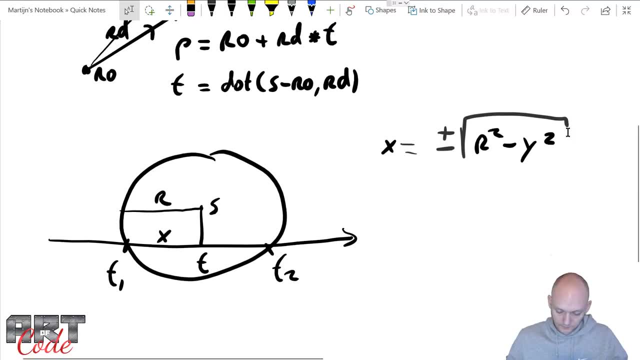 And whenever you do that, you have to take care that that's either plus or minus, Because if it's minus and you square it, then it becomes plus. So that's for my x. Now we already have the, the radius here, but we don't have this value yet. 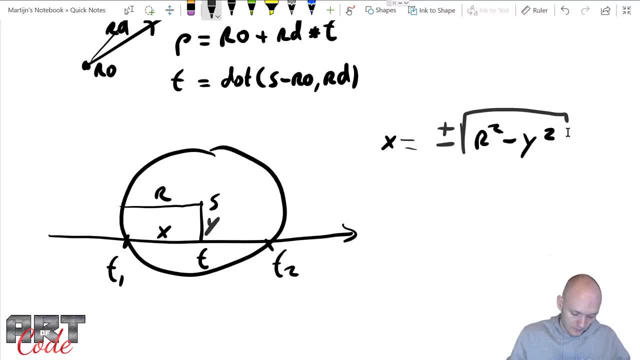 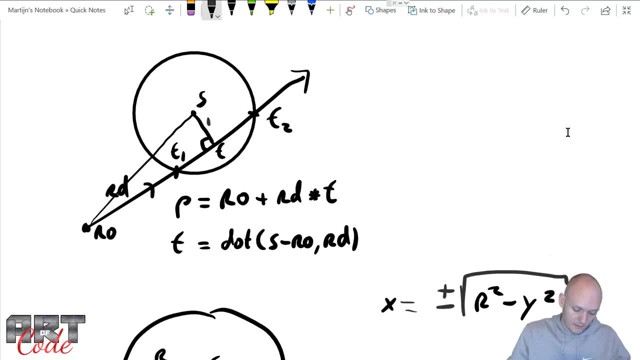 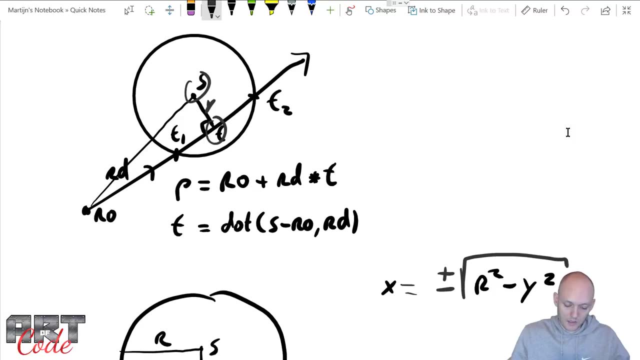 This y. And what is this y? Well, the y is basically over here, Okay, so, and what? what is the y if we go back to over here? So my y would be there, right? So my y is just the distance between this point s and this point described by by t. 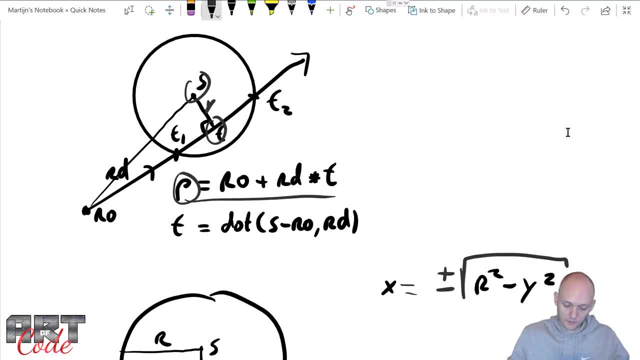 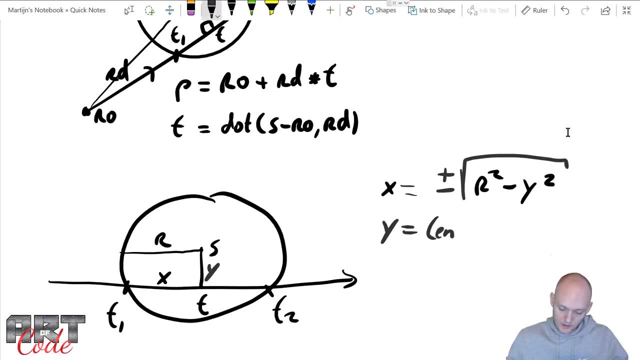 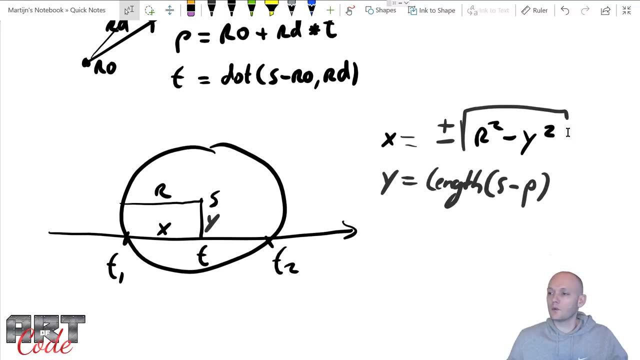 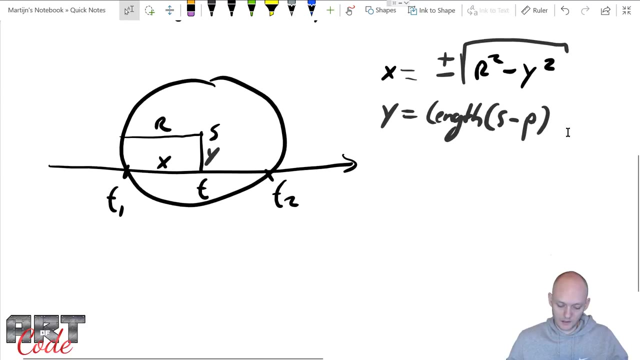 which is actually found by using this formula. So let's do that. So the y turns out to be the length Of s minus p. All right, So now we have. Now we have all the things that we need to calculate our t's, our t1 and t2.. 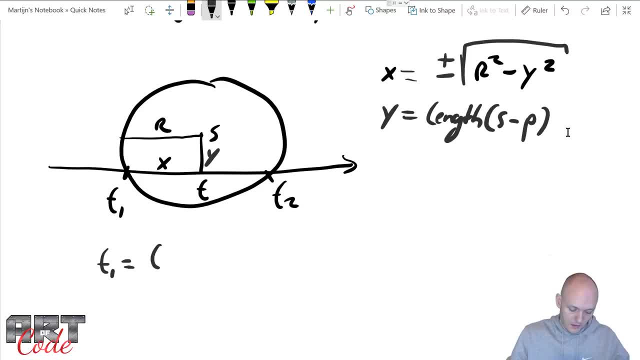 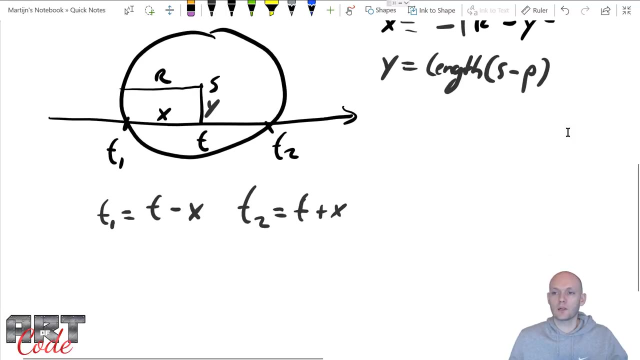 Because t1 is just t, right This t minus x, right That x, And t2 equals t plus x. Okay, so that is how we find the intersection on a sphere. So now let's try to implement this in shader toy. 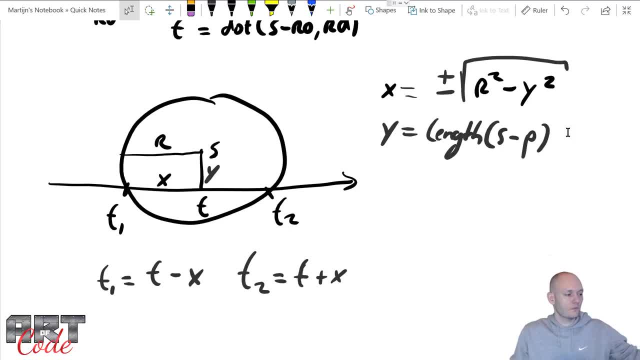 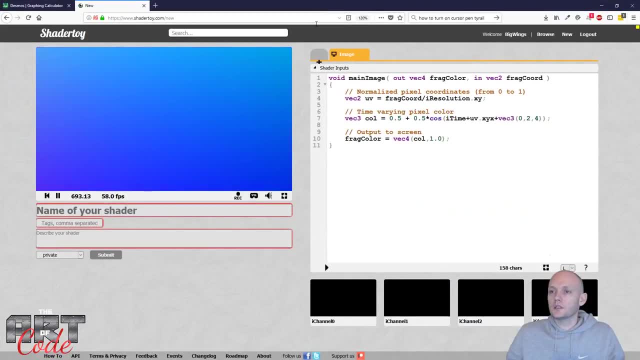 So let me put my tablet away And rearrange some stuff over here, And let's get shader toy. So there we go. So the first thing I have to do is: let's get rid of this. I have to normalize this a little bit more, because I want my UVs to be in the center of the screen. 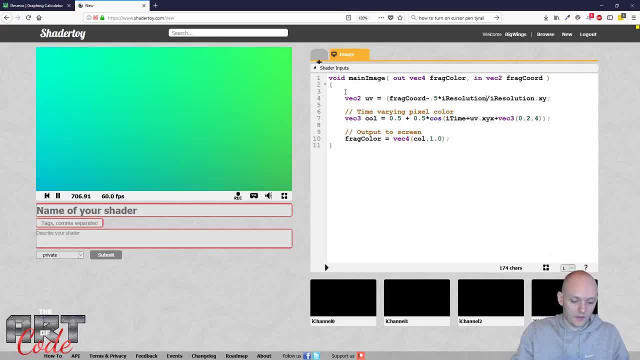 So I do that by subtracting half of the resolution, And then I just divide that whole thing by just the y instead of the xy, And then let's also get rid of all these fancy rainbow colors. So I'm just going to set my color to black. 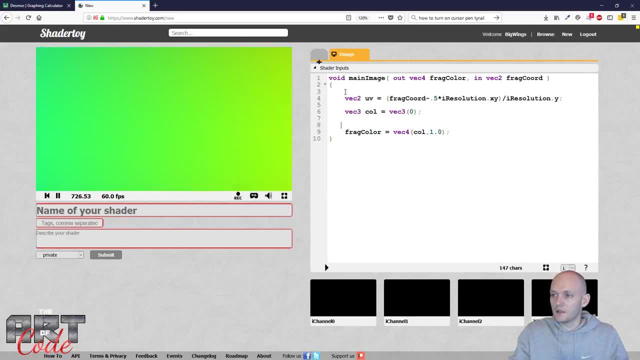 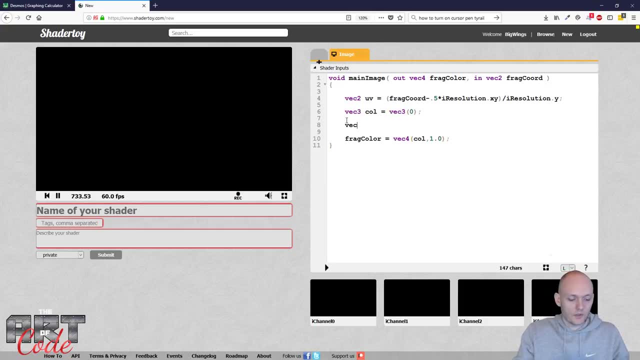 And let's get rid of this as well. All right, So there, we have a black screen. So now let's define some stuff. So first I'm going to find my ray origin, which I'm just going to keep it simple: Find it at zero. 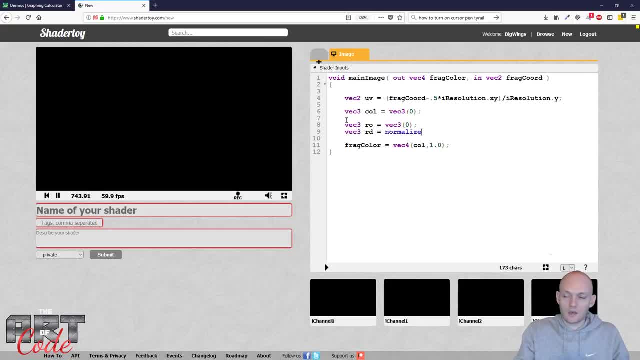 And then I'm going to make my ray direction, which I'm going to make a very, very simple camera model. If you don't know what I'm doing, check out this video. So that's vec3 uvx uvy 1.. 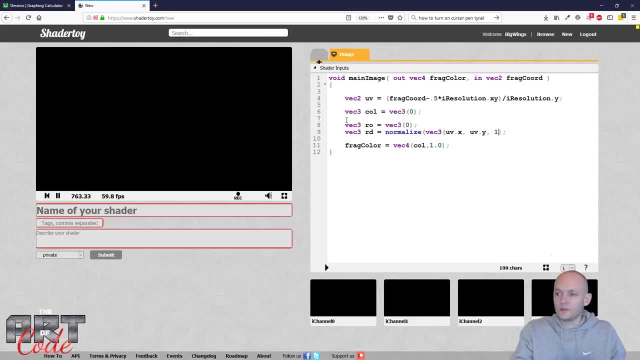 And then, All right, I need to Close my bracket And then I can define my point S, which is the center of the sphere, which I'm going to stick in the middle of the screen and then some distance away from us. 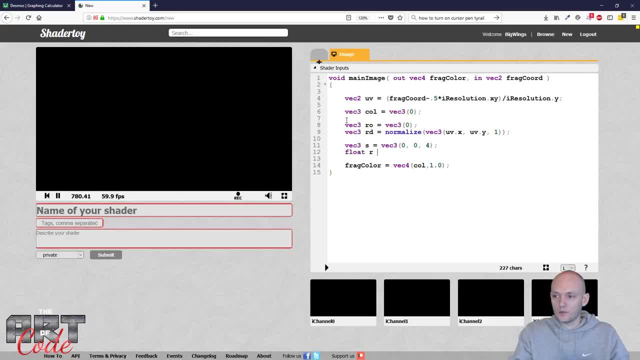 So let's say at four, And I'm going to define my radius. Again, keep it simple, Just one. All right, Now I can calculate my value t, So I'm going to do float. t equals A product of S minus the ray origin. 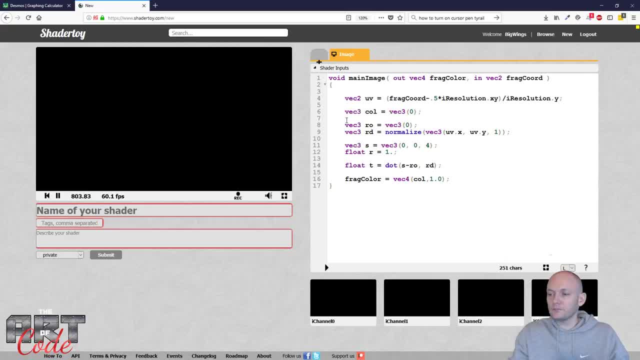 All right, And obviously the ray direction, And now I can do my y. So y equals the length of S minus p. Actually I have to get my value p that corresponds with the value t, So Ro plus rd times t. 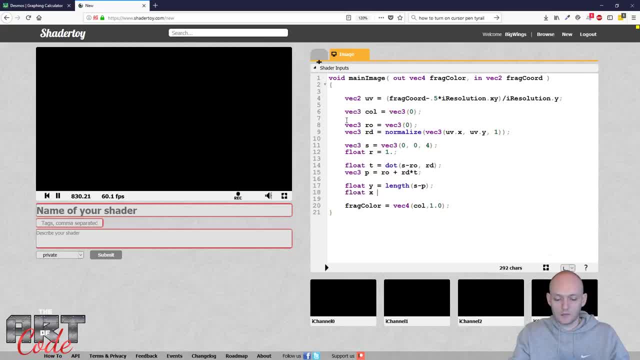 Okay, So now I have my y, Now I can get my x, So my x equals the square root of r times r plus, Not plus minus y times y. And now I can get my t, So t1 equals t minus x. 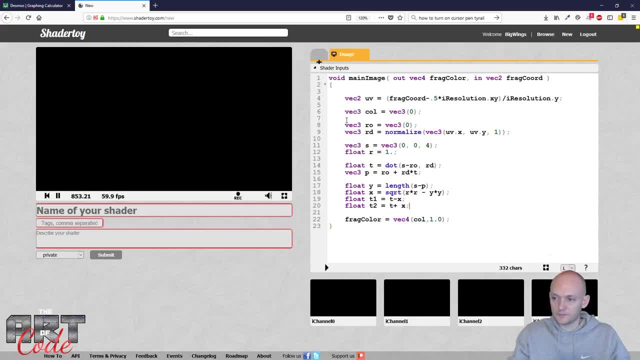 t2 equals t. t2 equals t plus x. And now there's one thing that I did mention, which is what happens when the ray doesn't hit the sphere at all, And what happens then is that my y value that I get is going to be larger than my radius over here. 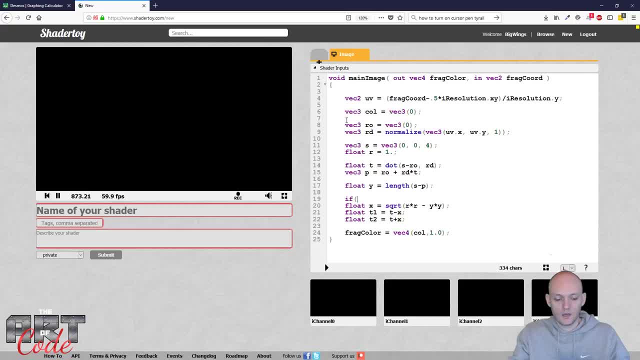 So I have to account for that. So over here I have to say: if This should only happen if the y is smaller than the radius, Then I should get in here, Because otherwise I'm wasting resources, because I'm not hitting the sphere anyways. 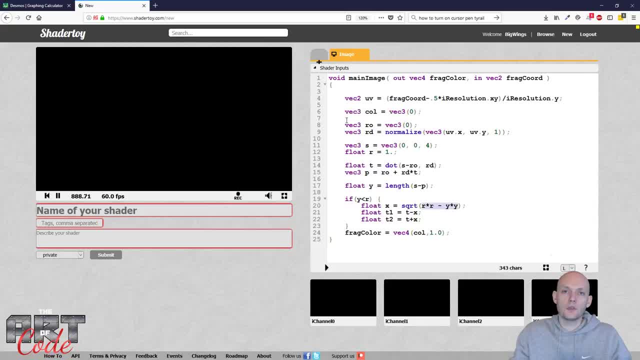 And plus this will become negative, which the square root of a negative number is going to be undefined. So that's why I put that in here, All right. So let's see, Let's keep it simple again. So let's say over here: col equals vec3.. 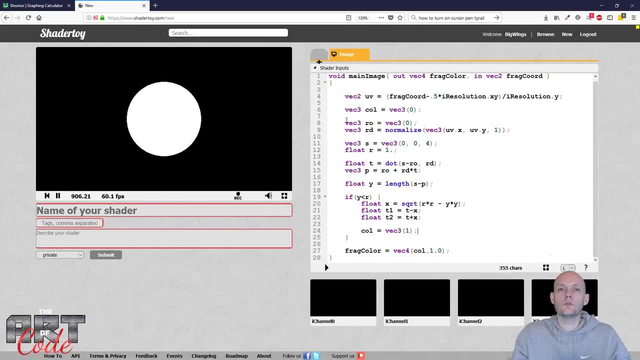 And then let's put it to white. So now that gives me a sphere, But I can use these values to color the sphere, Because these values are basically the distance from the origin, right From the origin to where it hits the sphere. 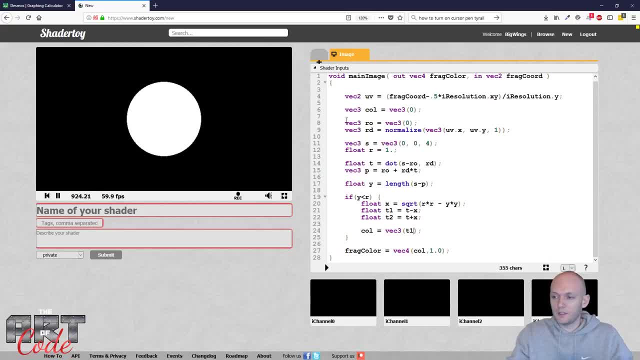 So I can say, okay, give me this t1 value. And here it still turns out to be white, Because let me drink something here for a second. Okay, Here it still turns out to be white because my t1 is larger than 1.. 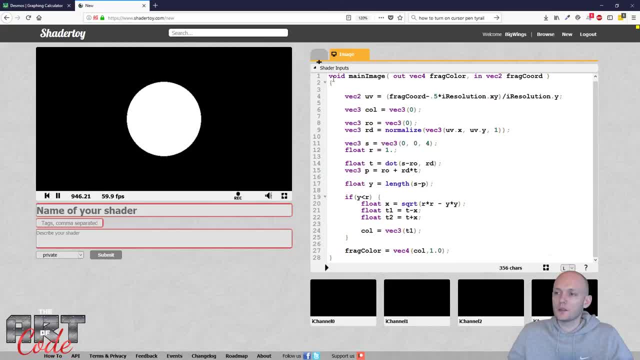 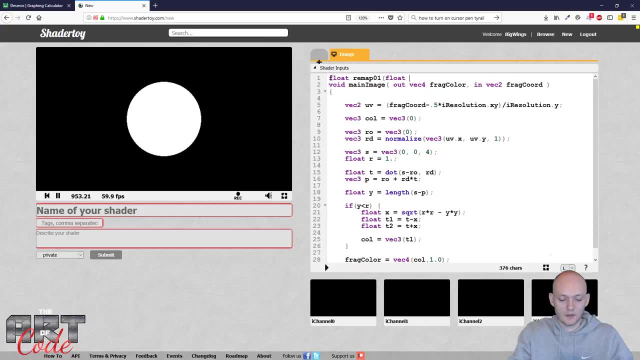 I have to remap it into the 0, 1 range. So for that I'm going to quickly make a function. Call it remap 0, 1.. It's going to take an input of float a, a float b and a float t. 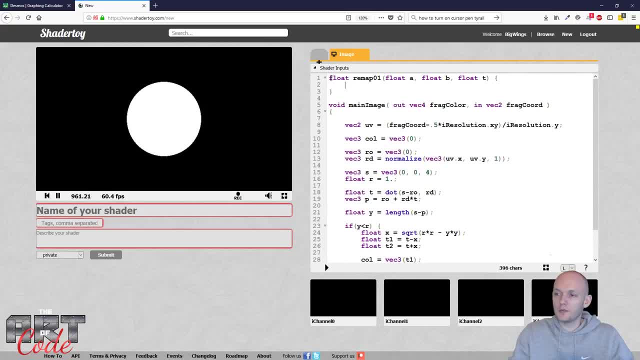 And that's just going to remap my number into a 0, 1 range that we can see. So for that I'm going to do this: t minus a divided by b Minus a, And what that will do is that if t is a, then it will return 0. 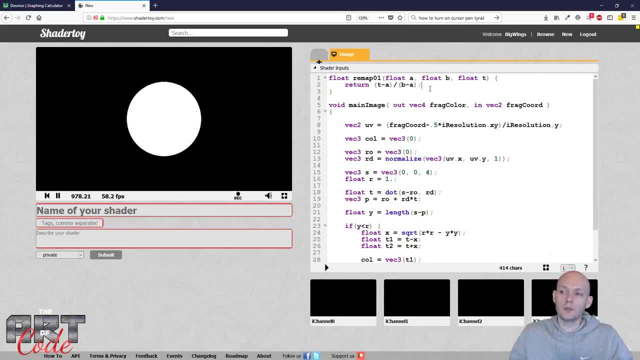 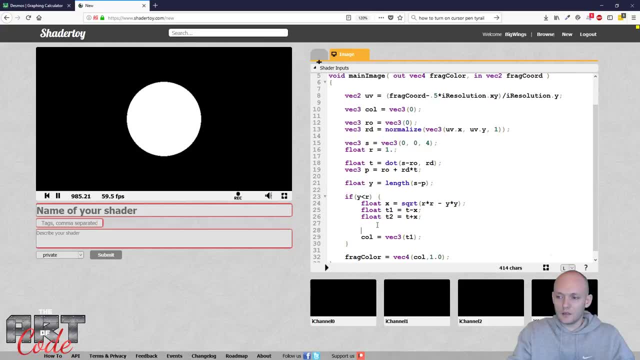 If t is b, it will return 1.. And anywhere in between it will return something in between. So now I can use that to make a value that we can actually see. So I'm going to do float c equals and then remap 0, 1.. 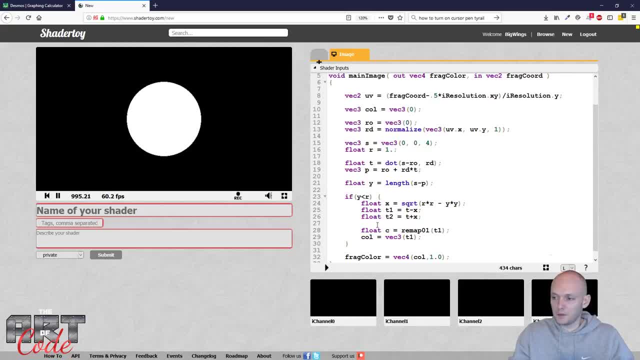 And then I'm going to remap this t1 value to something we can see. So for that, let's think about this. So we have the front of the sphere. here is basically the sphere center, the z position minus the radius. So that's s dot z minus the radius. 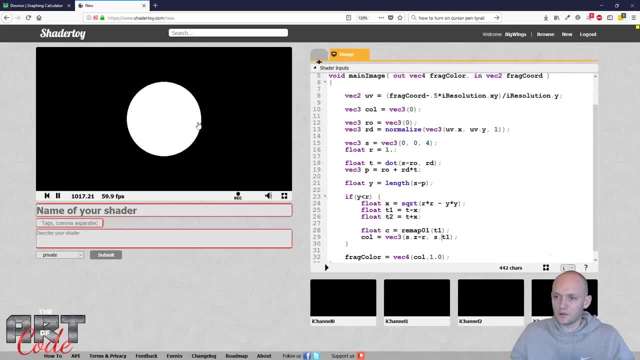 And then over here it's so over here on the edge it's just s dot z. So and obviously I put that in the wrong function, So I have to put that over here. And then over here I say c. 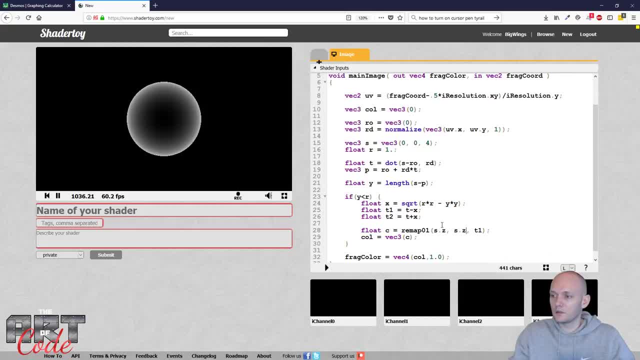 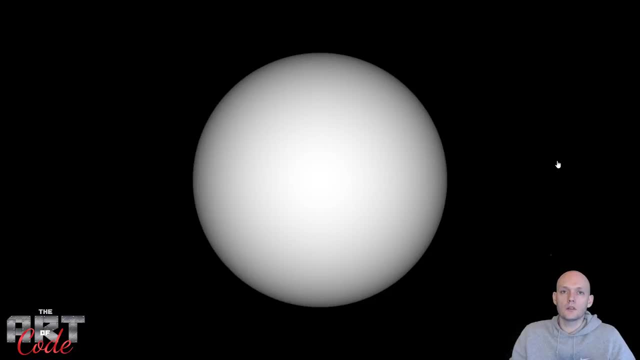 Okay, and now it did exactly the opposite of what I wanted. So let's just turn these around And we have a sphere, a shaded sphere, no less. All right, so let me put that full screen. So you might wonder, like, why go through all this trouble for a simple sphere intersection? 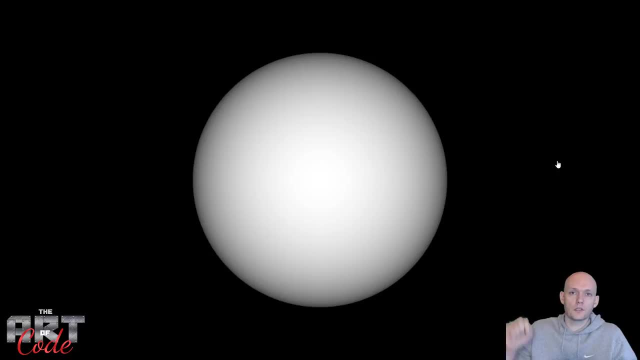 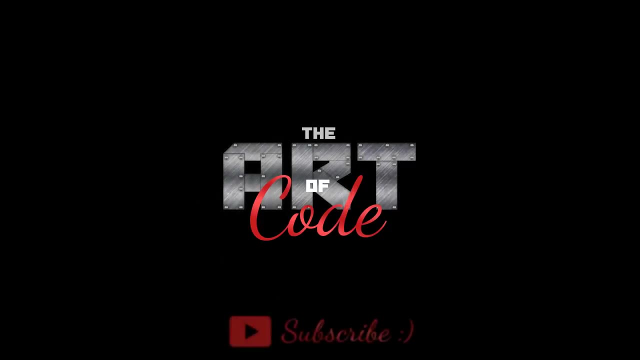 But you can make some pretty cool stuff with that. Check out this video, for instance. And either way, I will see you next time.